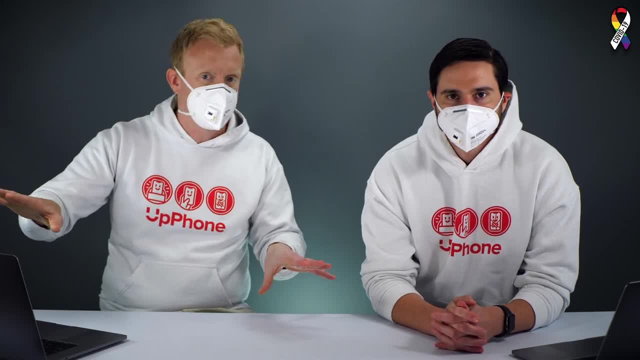 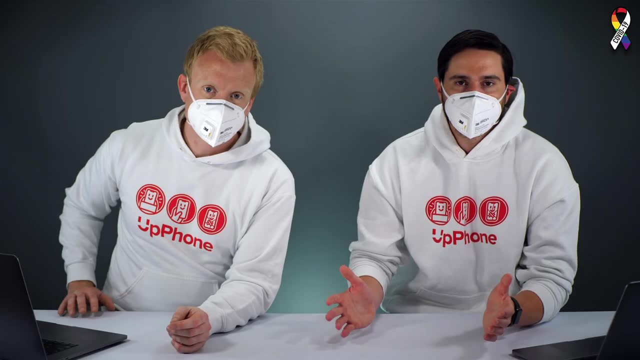 you need to make a good decision. So we didn't just exclude phones that we didn't like, but we did put a few of our favorites at the top. Yeah, So next is the capacity filter. How much storage space do you want your phone? 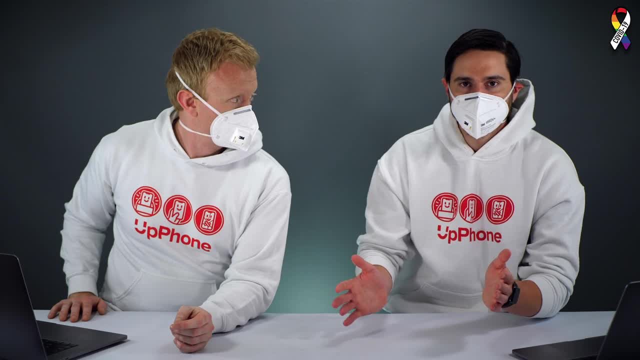 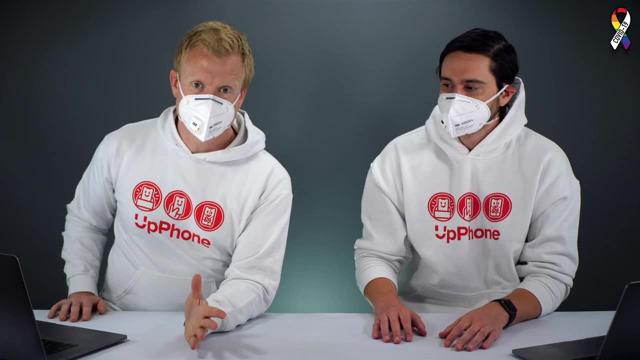 to have. I mean 64 is kind of the standard base model these days. Some older phones have 32 versions, 16 gigabyte versions, but 64 is enough for the average user. Yes, But if you're going to be taking a lot of 4K videos or 8K videos with the new Samsung, 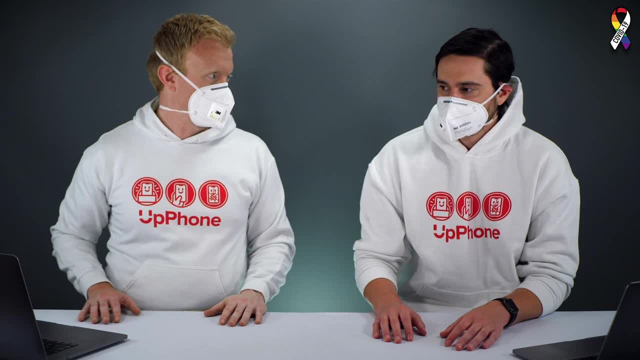 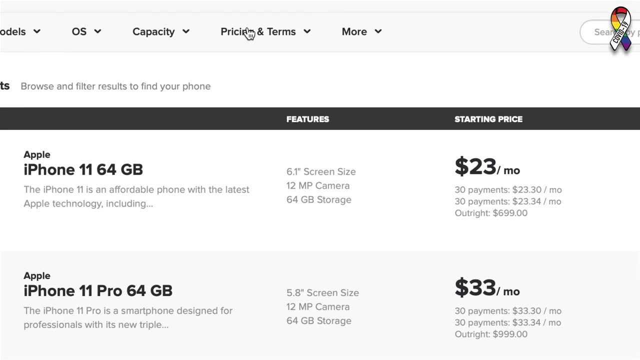 S20s, you might want to go more than 64.. Yes, 128,, 256,, all the way up to one terabyte. now, It's amazing. It's a lot, ton of storage, Yep. Next up is pricing and terms. What's your price range for your phone? What are? 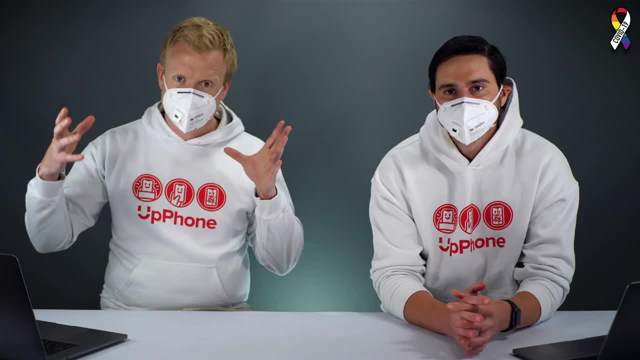 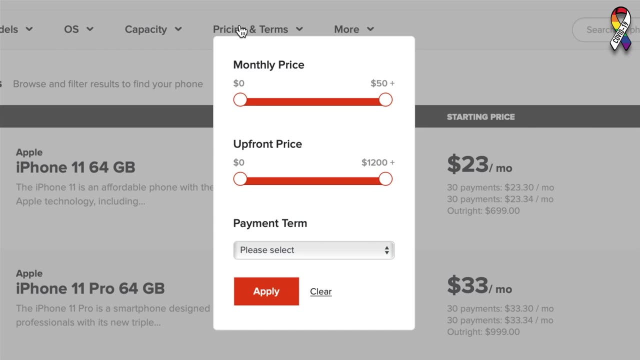 you comfortable paying outright or per month, Right? Do you want to just pay upfront? So we have this upfront price slider. You can do that And we have the monthly price slider. If you want to lease your phone through a carrier payment terms, you can choose lease installments, new line upgrade, et cetera. 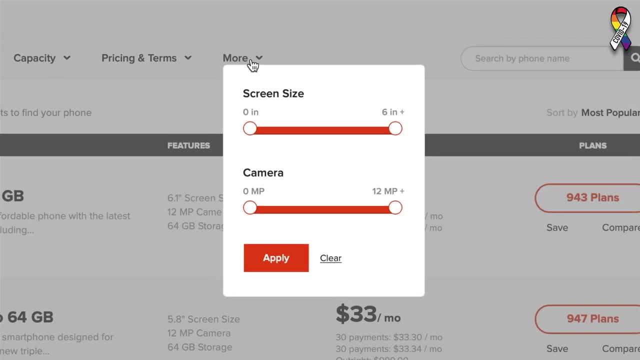 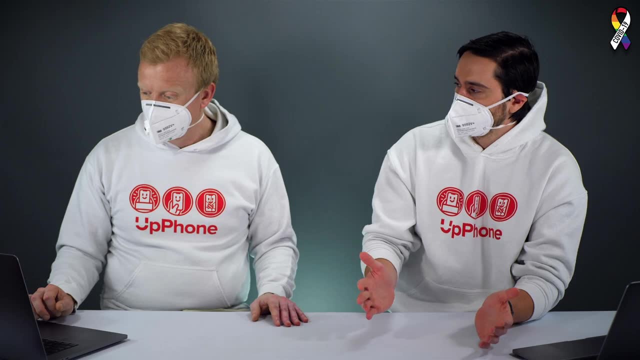 et cetera. And we have our nice more filters, screen size and camera. Do you want a big phone? Do you want a small phone? Do you want a really amazing camera, like the new Samsung Galaxy S20?, Or are you okay with a less than stellar camera? 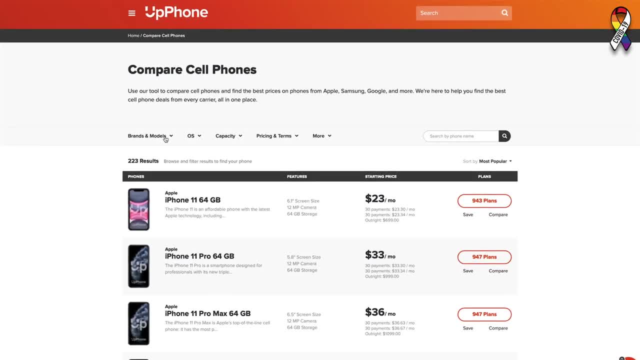 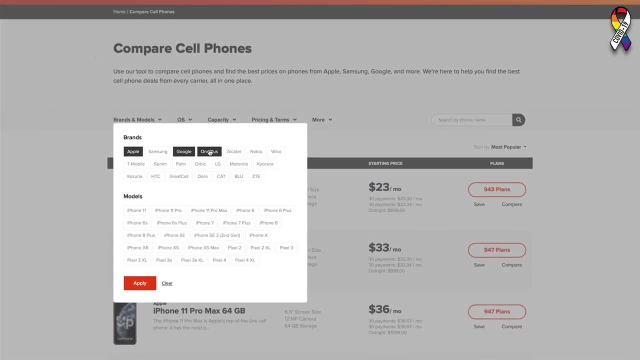 Yeah, So let's filter, Go ahead, All right. Let's say, I want to look at Apple phones and you don't have to choose specific models here, but you can Google phones and let's say OnePlus and LG, So you can either. 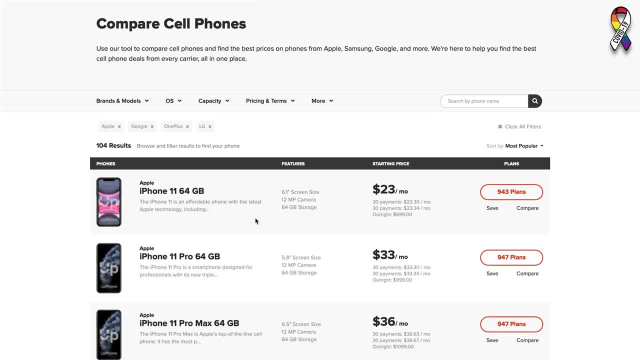 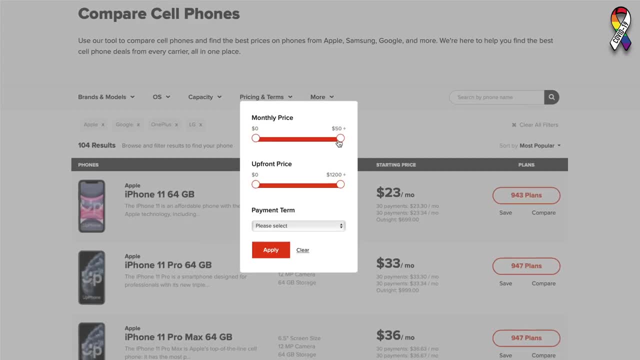 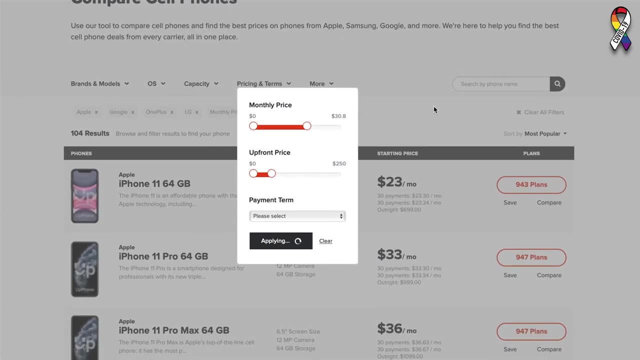 Yeah, We got a ton of results right there. We did Pricing and terms. Let's say I'm comfortable with a monthly price of 30 bucks. I don't want to have to pay much upfront. Let's say 250 max upfront. I'll say apply, All right. 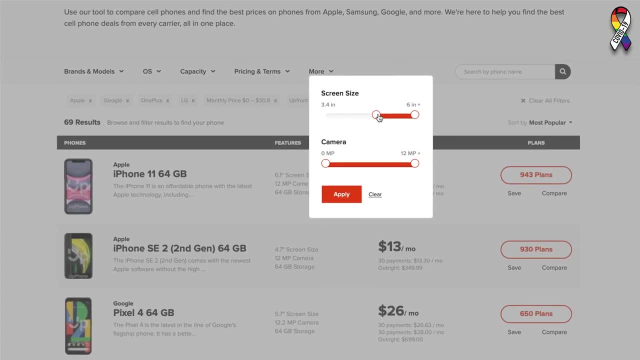 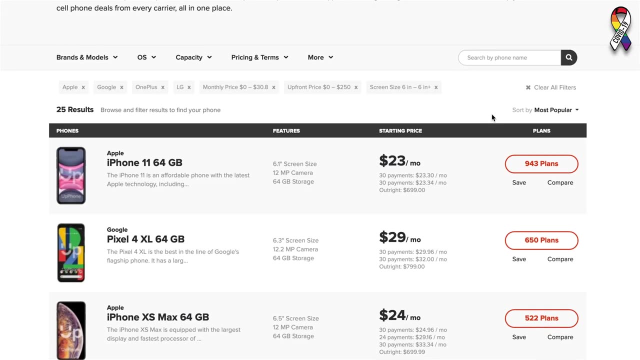 Filtered out more Now under more. I want to definitely have a screen size, Let's just say more than six inches. What do you say? Perfect, All right Click apply. We're down to 25 results. now, If you want to, you can sort by lowest price, highest. 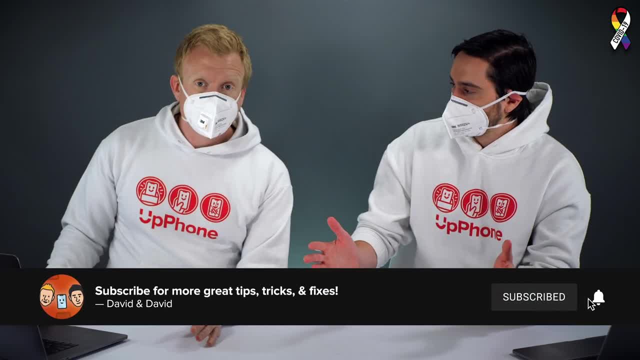 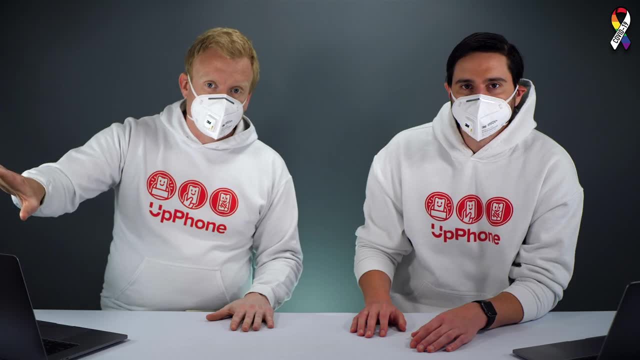 price. Mm-hmm, I don't know what the lowest price phone is. Maybe there's an older, cheaper budget iPhone that you like? Yeah, But we put every single phone in here, So sometimes there isn't as much information on phones that are very old. But again, we just wanted to make something real comprehensive. 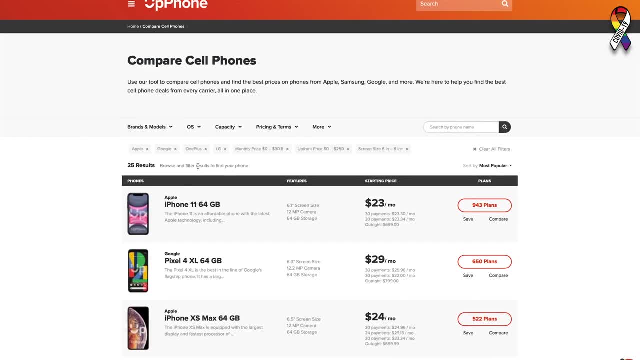 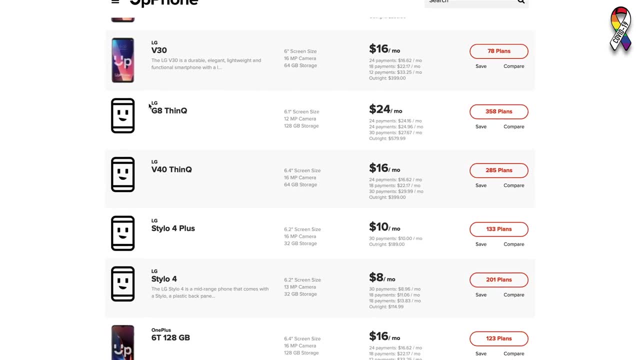 Could take a look through the list. We're down to 25 results already based on the filters that we selected, So I can just click load more. If you want to look at more phones, you can see here. these are some older phones that don't have pictures, but let's just focus. 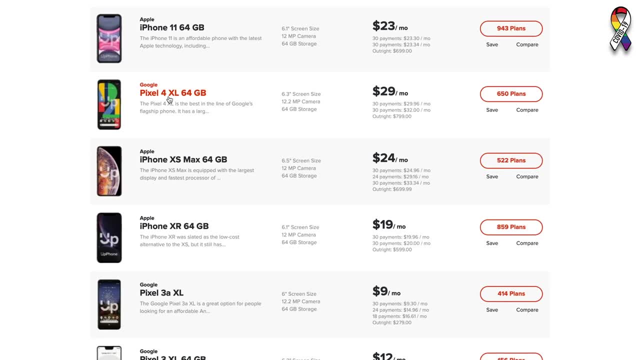 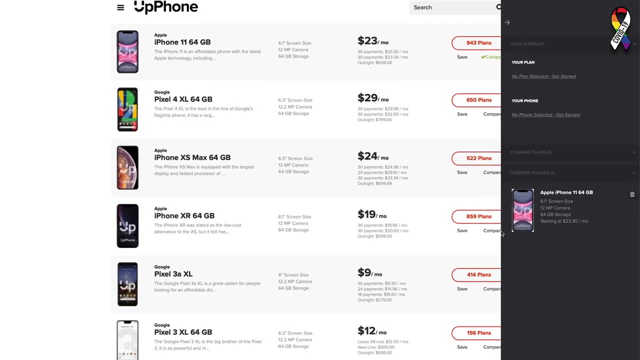 on what we find at the top here. So an iPhone 11 is a great phone. Google pixel four is also a great phone. We compare them head to head by clicking that compare button. All right, I'm going to click the compare button. Then it's going to pop out this drawer. 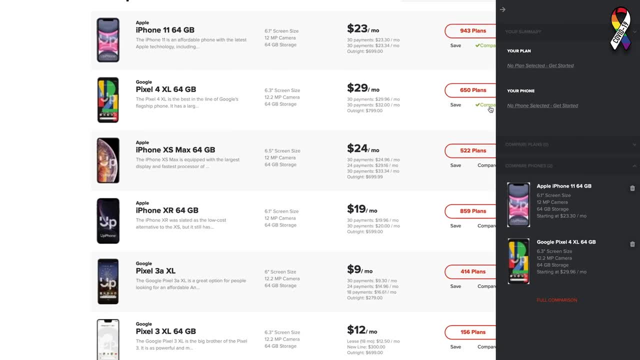 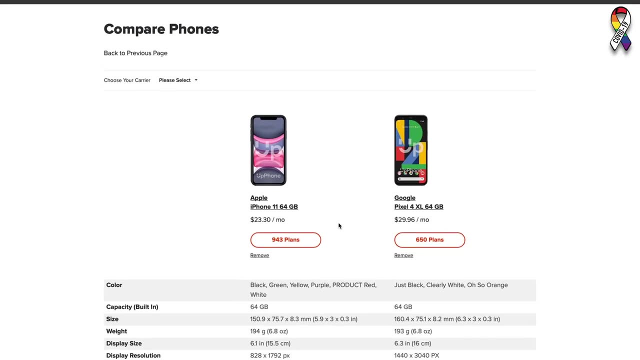 here. I can click out of it to close it, Click the compare button again and then click full comparison. This is going to put our two phones side by side, So on the compare page we can see the lowest price per month, And we're going to get to that in a second. You can. 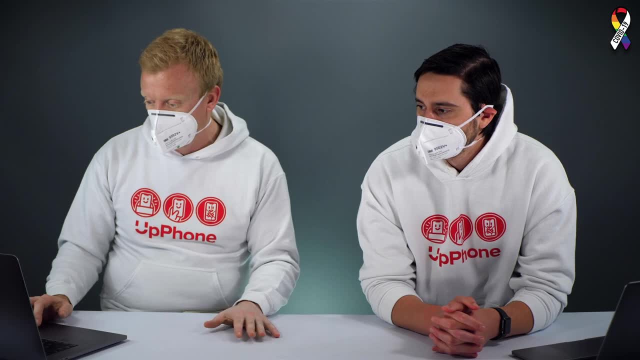 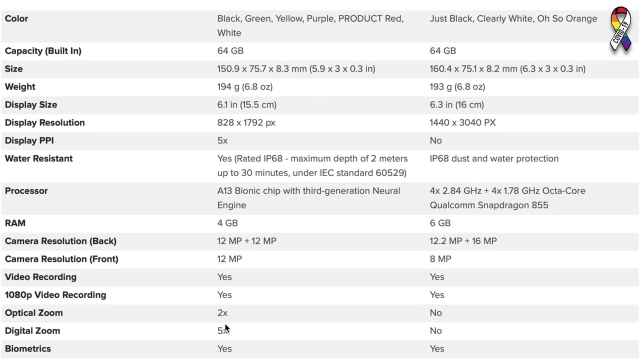 see every carrier's prices in the same place. It's awesome. You will not see that anywhere else online. The size, the way, display size and all the things that people really care about right here, head to head- Yep, That's the whole thing. So let's say we decided on the iPhone 11.. What's our next step? Let's 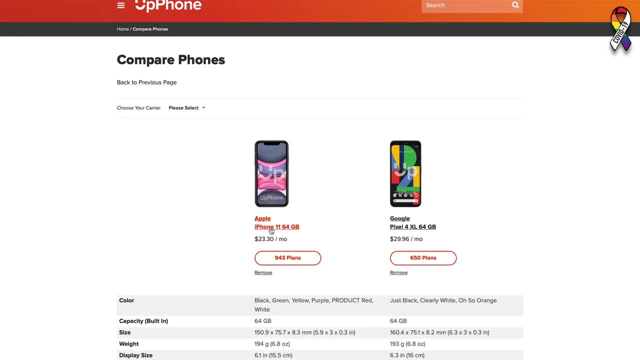 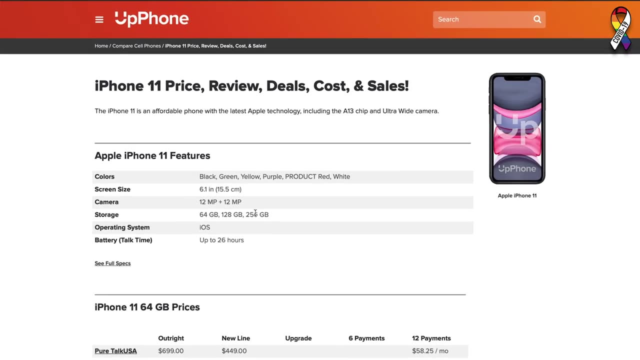 click right here where it says Apple iPhone 11 64, or I can just go back and click right where it says Apple iPhone 11 64.. So let's take a look The top of the page. we have some features that you care about the most. We asked people in our Facebook group and 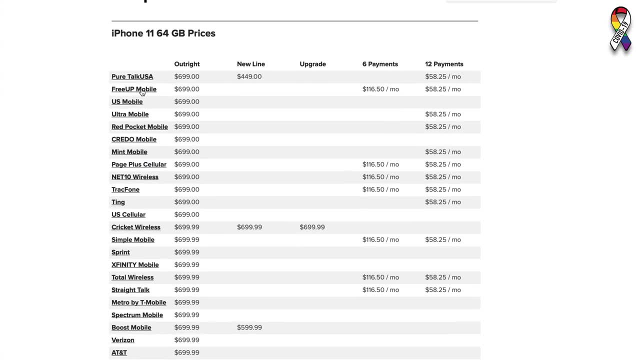 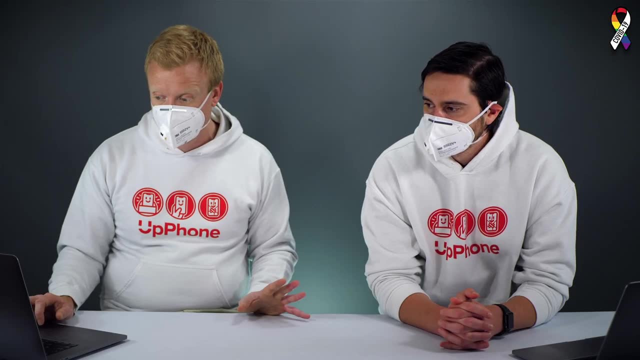 this is really cool. iPhone 11: 64 gigabyte prices on every single carrier with every single payment term. Now this looks like a lot, but it's going to be very useful for you. Yeah, As you can see here, PureTruck USA. if you get a new line through them, you can get the. 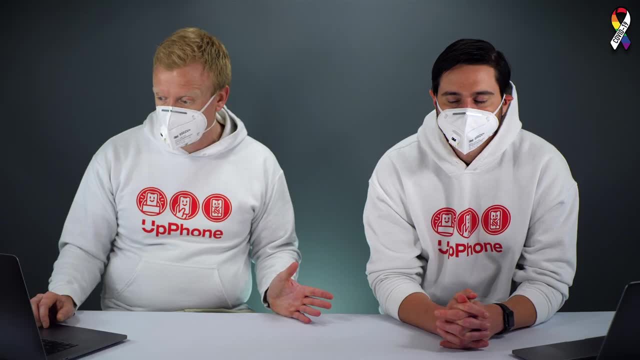 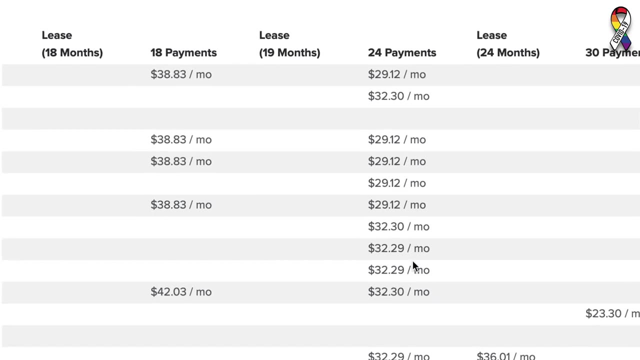 phone for 450 bucks, which is a lot cheaper than anybody else. So six payments, 12 payments is a pretty common payment term. 18 or 24 payments is also pretty common. If I scroll down, I can see the other variants of this phone. So there's 128 gigabyte version and 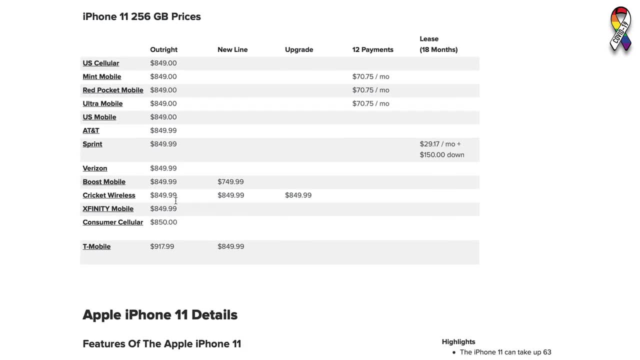 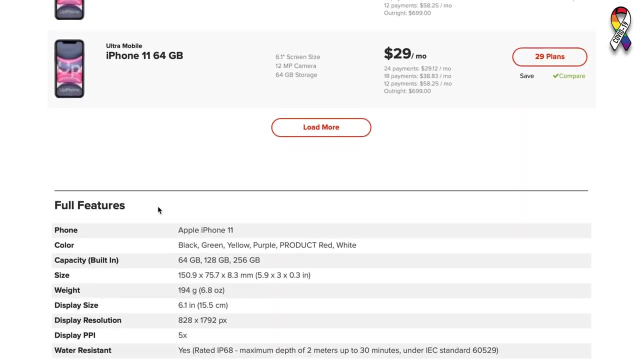 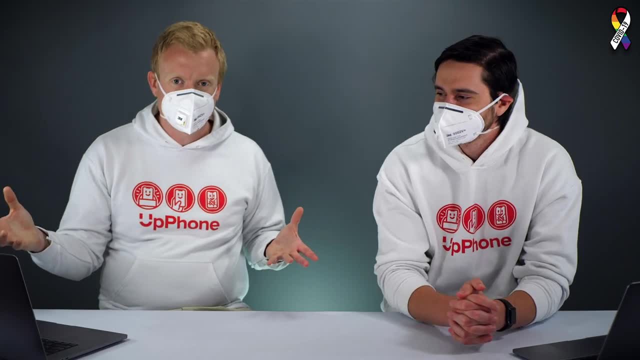 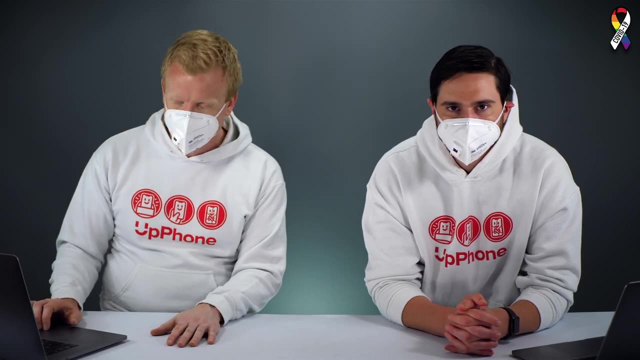 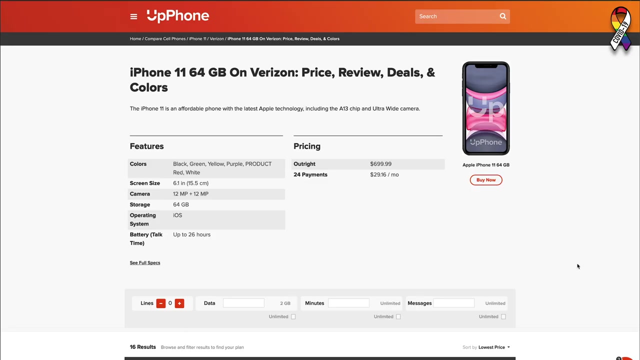 different phone reviews. Yeah, it's not just auto generated stuff. This is stuff that we've actually written, and we also have other people that write for us as well, but David is the editor in chief. let's say So. let's say we wanted to check out this phone on Verizon after looking at the prices And 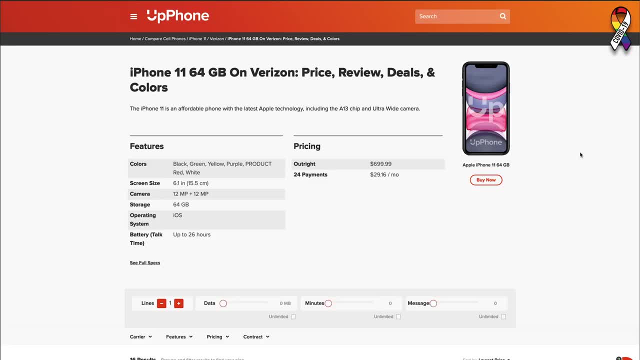 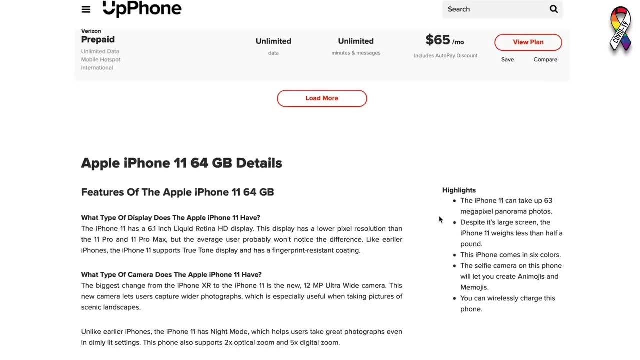 now we see iPhone 11- 64 gigabyte of Verizon price review deals. if you're thinking about switching carriers when you're buying a new phone, these pages also have a coverage map at the very bottom where you can just check to see if this carrier has good coverage. 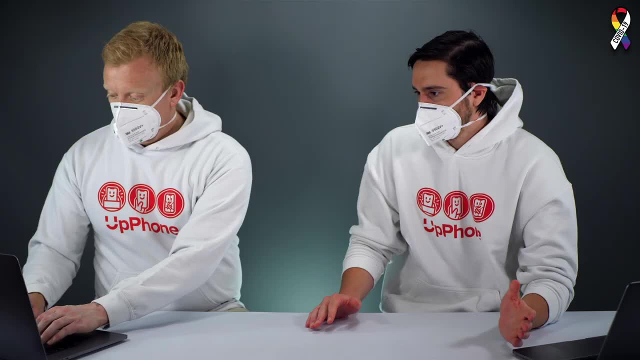 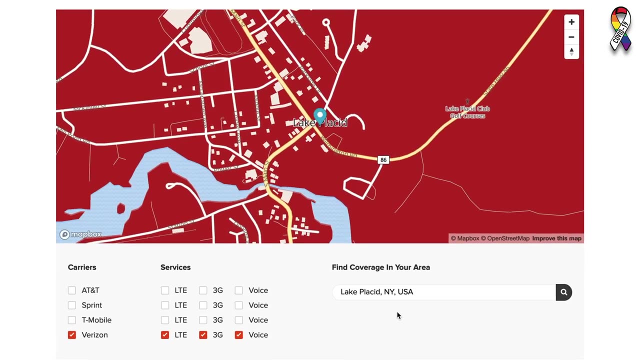 in your area because you don't want to buy a new phone locked on a carrier's network, and then it turns out they don't have coverage in your area and you're just. it's a whole mess. A useful tip here is to make sure to check your favorite vacation spots too, not just where you live. 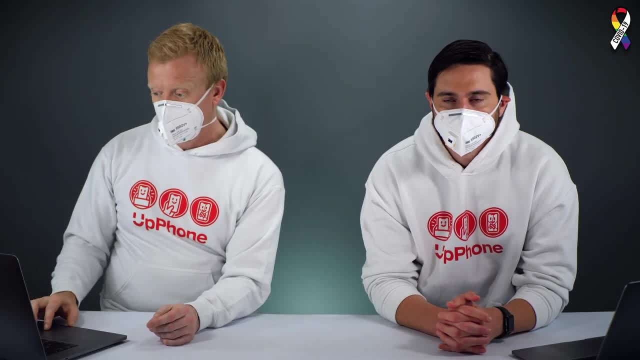 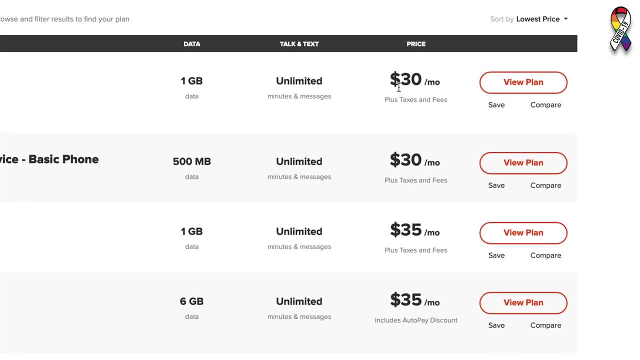 because a lot of times vacation spots are more out in the middle of nowhere than homes. Let's take a look at the Verizon plans that they offer for this phone and this prepaid plan, with one gigabyte of data for 30. There's a six view byte version, which I actually have, for 35, so I'm just 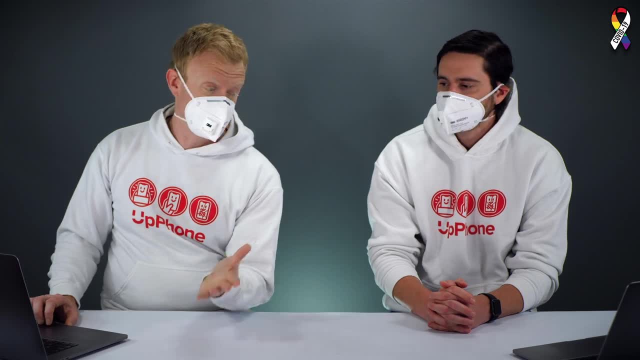 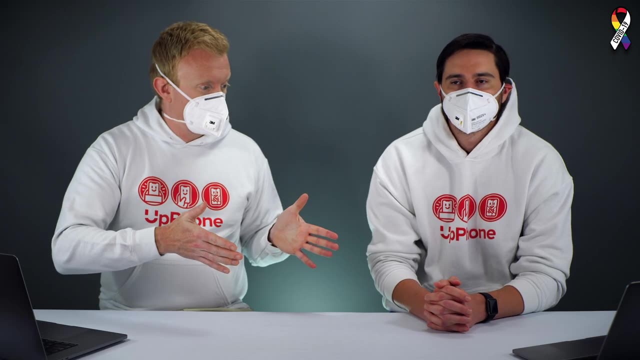 going to click view plan. You can read about the plan too. David also did an amazing job writing reviews for every plan and if you're ready, click- go to website. So what we found is that we can get the phone- an iPhone 11- for about 30 bucks a month on Verizon, and then you get the plan for 35 bucks. 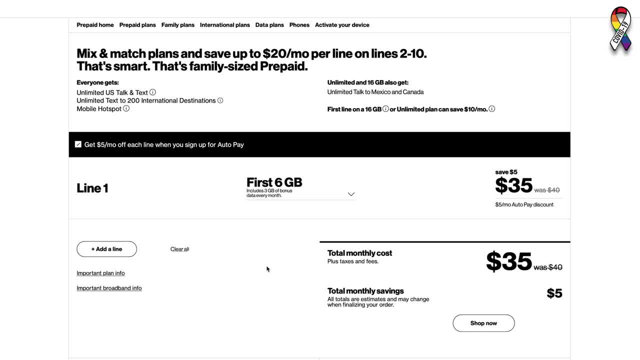 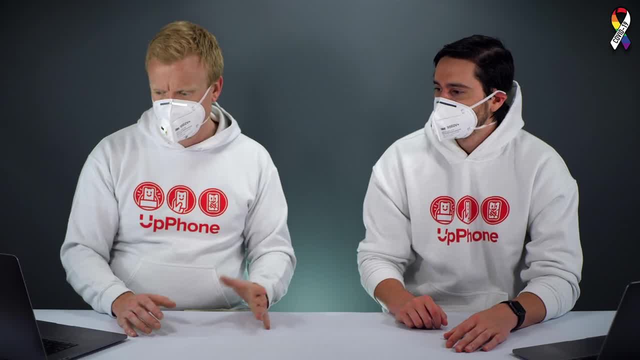 a month on Verizon. So you're going to be paying 65 dollars per line for the phone. A new iPhone 11.. That plan also includes mobile hotspot. I have the same plan too. It's a great plan. It is a great plan and I mean, come on 65.. A lot of people are paying just that much for an. 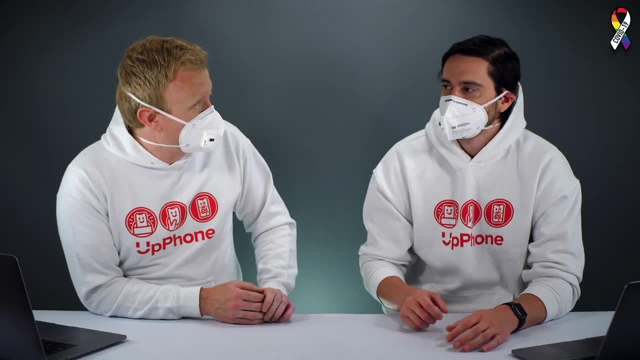 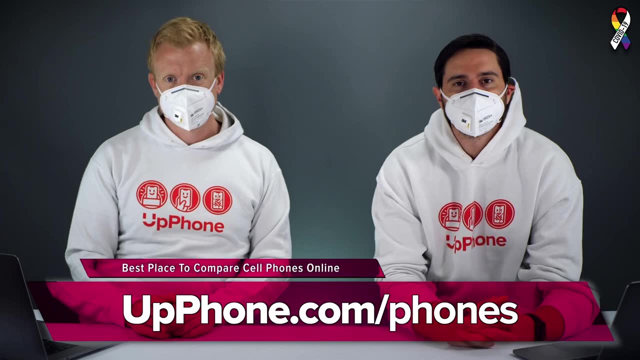 unlimited data plan that they probably don't need, and we've put out some other videos that we can link to that are really going to help you save money on your cell phone bill- Absolutely. so that's how to compare cell phones online. Thanks for watching this video. Give it a thumbs up if. 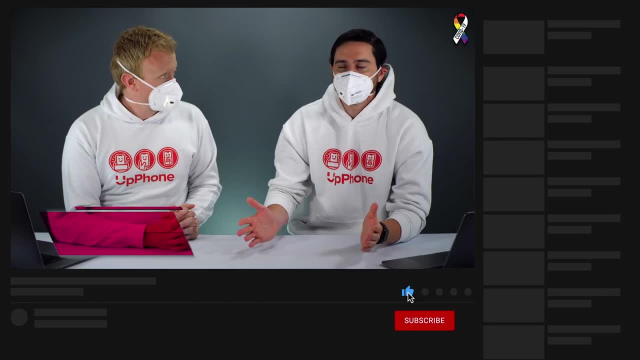 you enjoyed. Leave us a comment down below, if you have any, you know, looking for phone recommendations maybe, or have a question about your phone? and don't forget to subscribe to the this channel for more great videos about cell phones and plans.